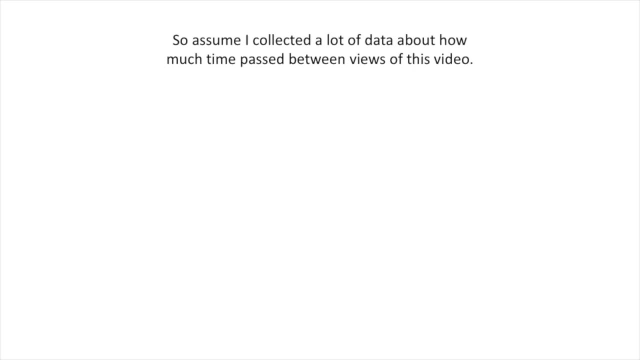 collected a lot of data about how much time passed between views of this video. X sub 1 equals the amount of time that passed between the first and second views. X sub 2 equals the amount of time that passed between the second and third views. X sub 3 equals the amount of. 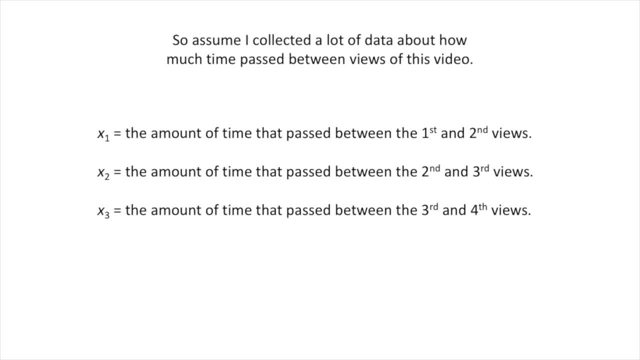 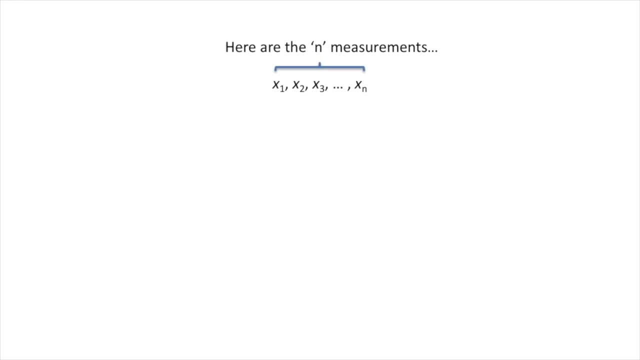 time that passed between the third and fourth views, etc. etc. etc. Here are the n measurements. For now. let's assume we already have a good value for lambda. What's the likelihood of lambda, given our first measurement, X sub 1?? Here's the likelihood. 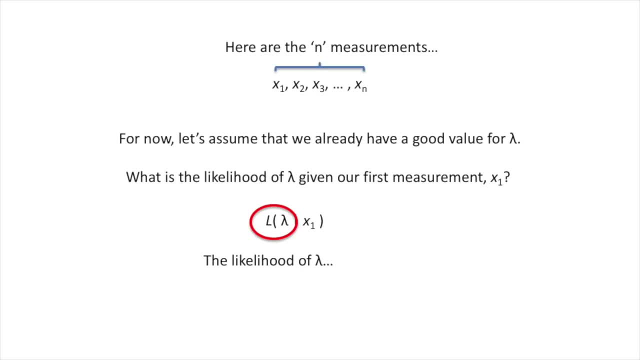 function, We have the likelihood of lambda, given that we have this measurement, X sub 1, and the likelihood equals this equation. This equation is just the equation for the curve, with X sub 1 plugged into it. If X sub 1 was here, the likelihood of lambda would be this value on the y-axis. 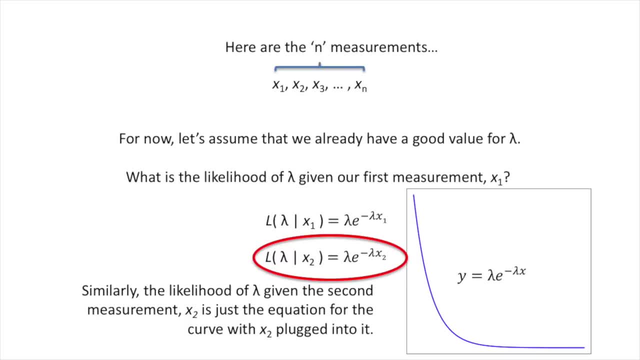 Similarly, the likelihood of lambda given the second measurement, X sub 2, is just the equation for the curve. with X sub 2 plugged into it, The likelihood of lambda would be this value on the y-axis. What is the likelihood of lambda given both x sub 1? 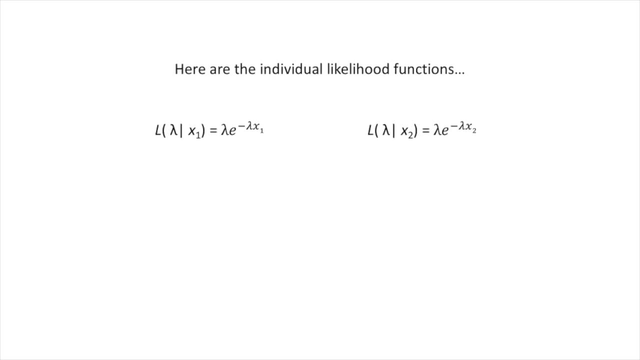 and x sub 2?. Well, here are the individual likelihood functions and here's the combined likelihood function. Because we are interested in x sub 1 and x sub 2, we multiply the two likelihood functions together Here I've just plugged in the two likelihood equations. 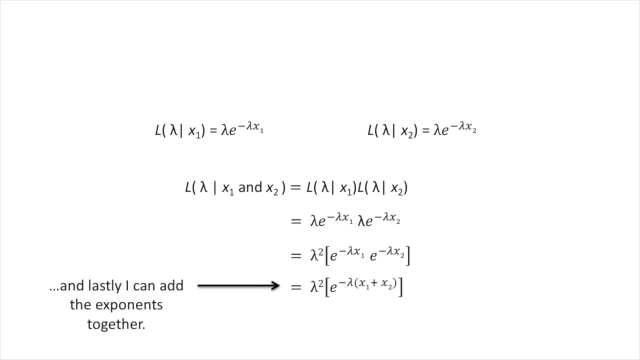 And now I've pulled the two lambdas out. And lastly, I can add the exponents together. Thus, this equation is the likelihood of lambda, given x sub 1 and x sub 2.. BAM, What is the likelihood of lambda, given all of the data? 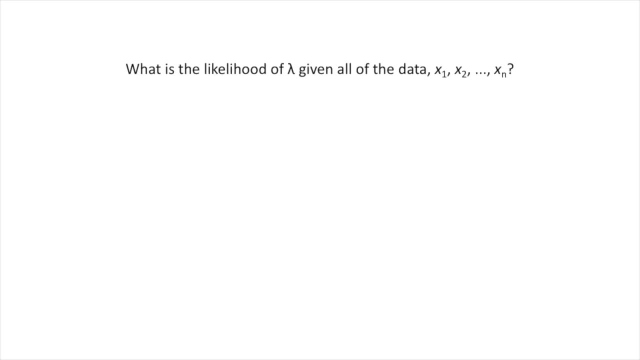 x sub 1, x sub 2, all the way to x sub n. Here's the likelihood function that includes all of the data we have collected. It is equal to the product of all the individual likelihoods Here. I've just plugged in all the individual likelihood equations. 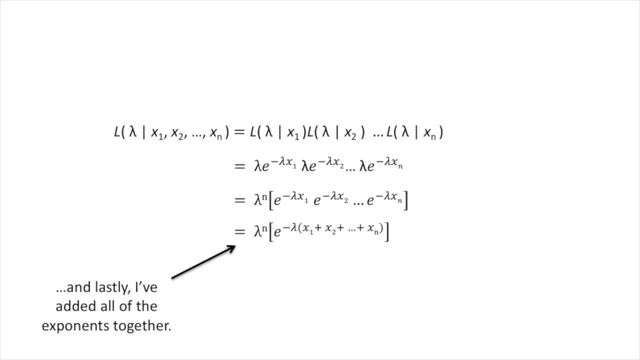 And now I've just pulled out all of the lambdas And lastly, I've added all of the exponents together. Thus, this equation is the likelihood of lambda, given all of the data: x sub 1,. x sub 2,. 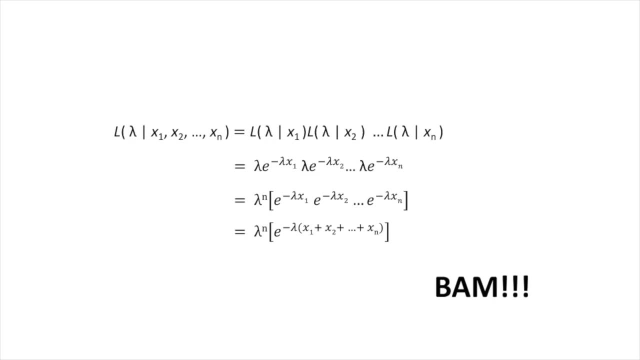 all the way to x, sub n, BAM. What if we don't have a good value for lambda? Well, we try different values for lambda to find a good one, To find the maximum likelihood. we one take the derivative of this. 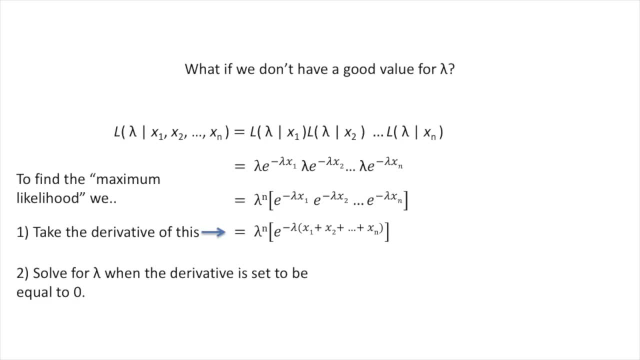 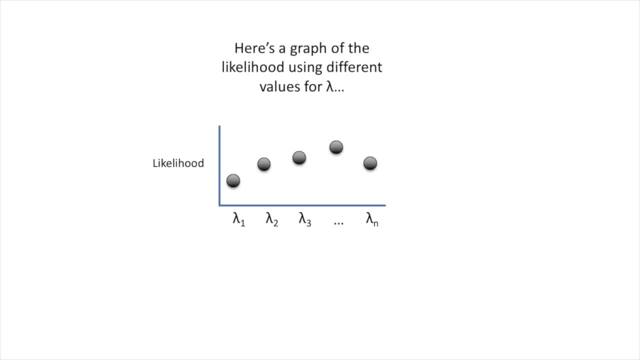 and two solve for lambda when the derivative is set to be equal to zero. Here's a graph of the likelihood using different values for lambda. At the maximum likelihood, the slope and thus the derivative will be equal to zero. 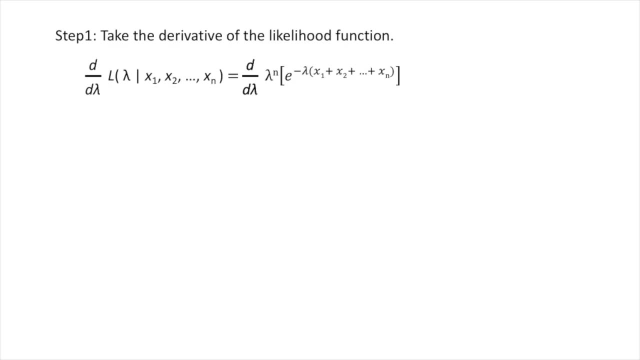 To find the maximum likelihood estimate for lambda, step one, we take the derivative of the likelihood function. Any time you have a function with a function, with a function, an exponential in it, it's almost always easier to take the derivative of the log of that function. 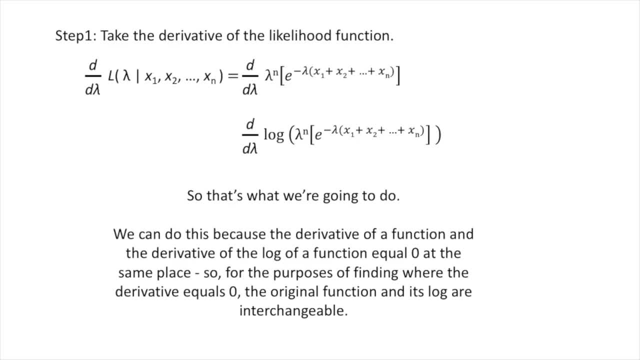 So that's what we're going to do. We can do this because the derivative of a function and the derivative of the log of a function equals zero at the same place. So, for the purposes of finding where the derivative equals zero, the original function and its log are interchangeable. 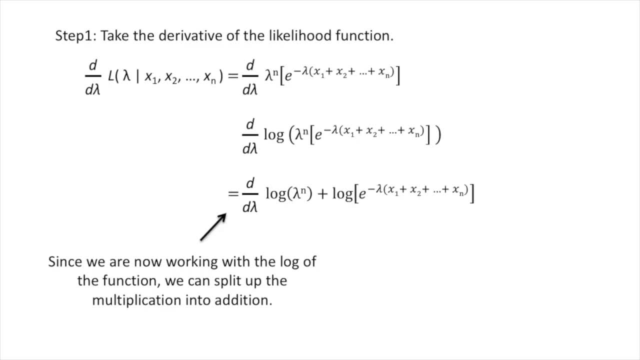 Since we are now working with the log of the function, we can split up the multiplication into addition. Next we move lambda's exponent n to be in front of the log, And the log of the exponential function reduces to just its exponent. 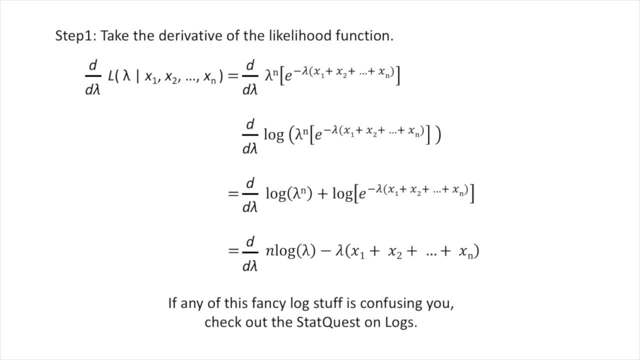 If any of this fancy log stuff is confusing, you check out the StatQuest on logs. Finally, we take the derivative of a function and the derivative of a function n to be in front of the log. Finally, we take the derivative of a function and the derivative of a function n to be in front of the log. 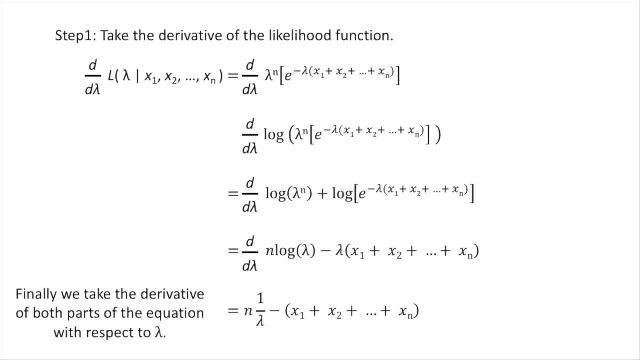 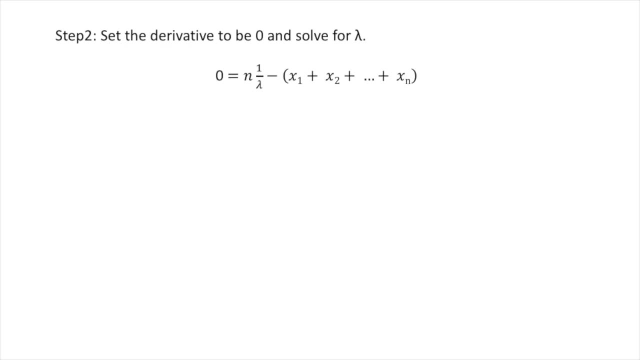 Finally, we take the derivative of both parts of the equation with respect to lambda. Now we move on to step 2.. Set the derivative to be zero and solve for lambda. Here I added x sub 1 plus x sub 2 plus all the way to x sub n to both sides, causing the term to cancel out. 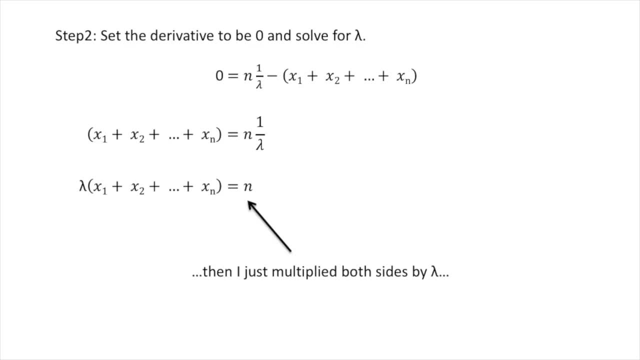 on the right side of the equal sign. Then I just multiplied both sides by lambda, And last I divided both sides by x sub 1 plus x sub 2 plus all the way to x sub n. This is the maximum likelihood estimate for lambda Double bam. 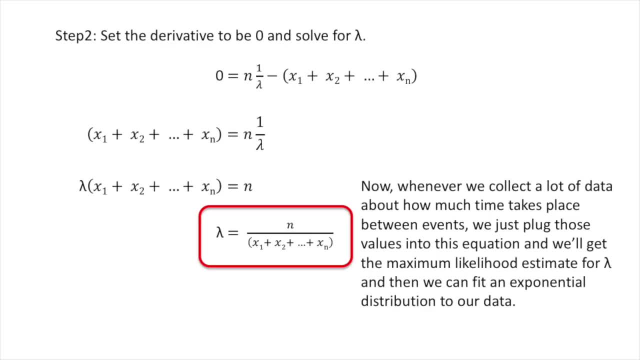 Now, whenever we collect a lot of data about how much time takes place between events, we just plug those values into this equation and we'll get the maximum likelihood estimate for lambda, And then we can fit an exponential distribution, which is the number of times that we can see a video. 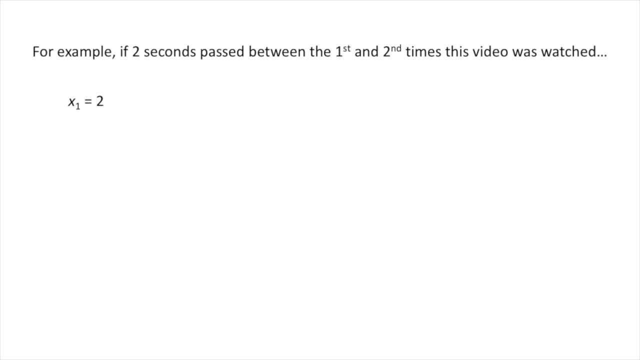 For example, if two seconds passed between the first and second times this video was watched, then x sub 1 would equal 2.. And if 2.5 seconds passed between the second and third times this video was watched, then x sub 2 would equal 2.5.. And if 1.5 seconds passed between the third and. 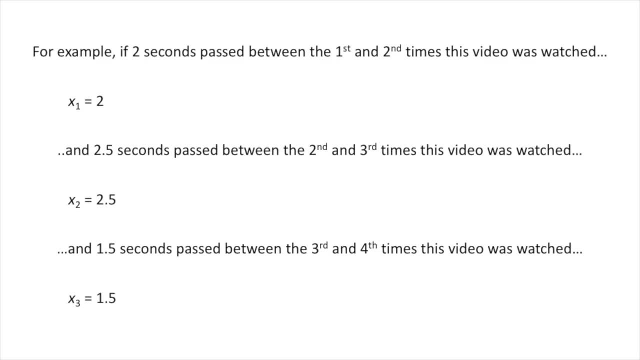 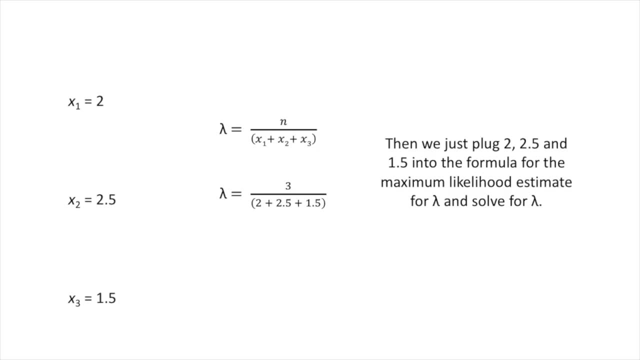 fourth times this video was watched, then x sub 3 would equal 1.5. Of all our data. we just plug in 2, 2.5, and 1.5 into the formula for the maximum likelihood estimate for lambda and solve for lambda. 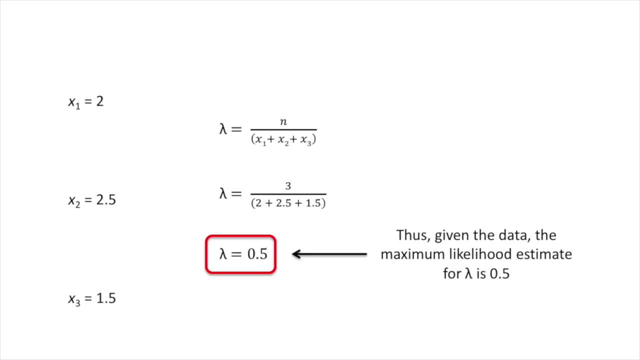 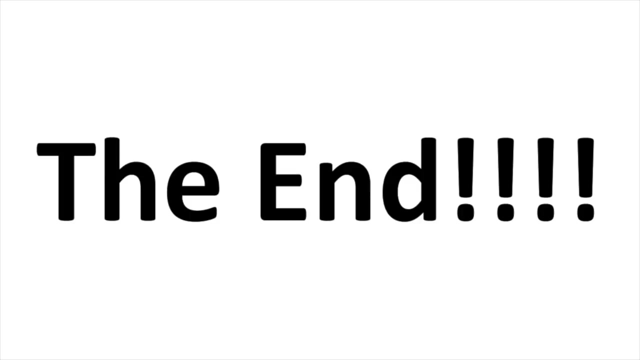 Thus, given the data, the maximum likelihood estimate for lambda is 0.5.. And this is what an exponential distribution looks like when lambda equals 0.5.. Hooray, Hooray, Hooray, We've made it to the end of another exciting StatQuest. 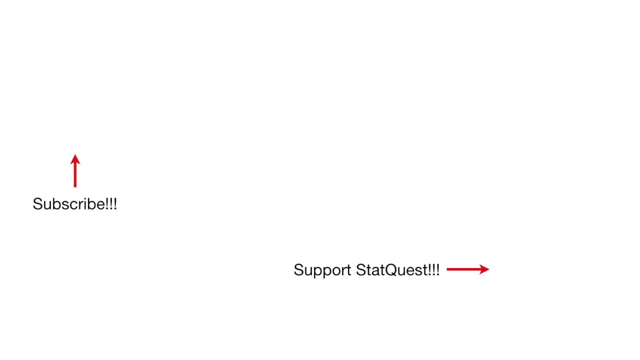 If you like this StatQuest and want to see more well, please subscribe. And if you want to support StatQuest, please click the like button below and consider buying one or two of my original songs. Alright, until next time. quest on.